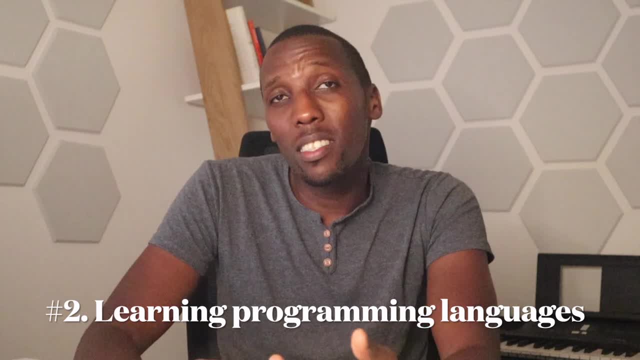 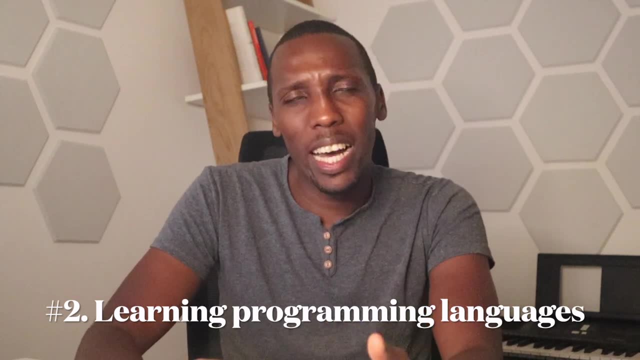 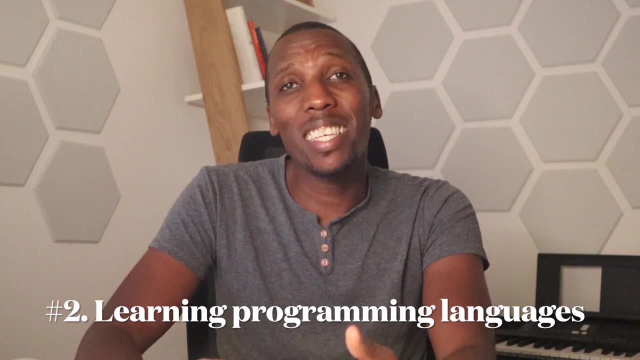 programming languages such as R or Python is essential for working with large data sets, considering that, most of the time, you're going to be working with a lot of data as a health data analyst, And these programming languages are commonly used in data analysis and can be helpful in the analysis of your work, as well as the creation of. 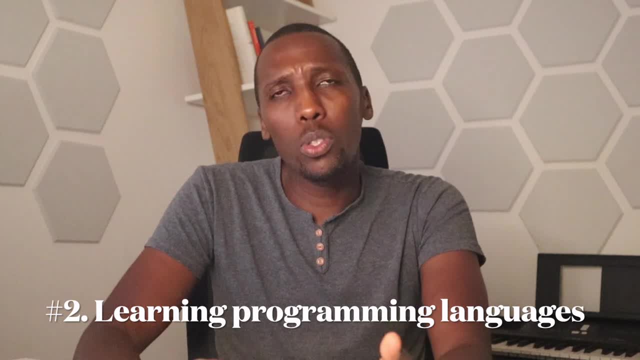 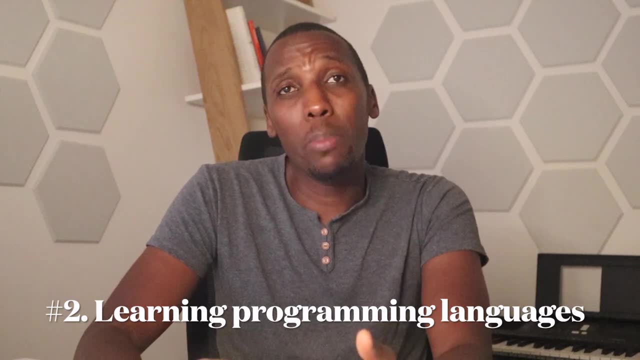 visualizations which you would present, which you'd use in presentations or reports to other stakeholders. So you can start by learning the basics of programming and then move on to more advanced topics such as data visualization and machine learning, as you start your journey. 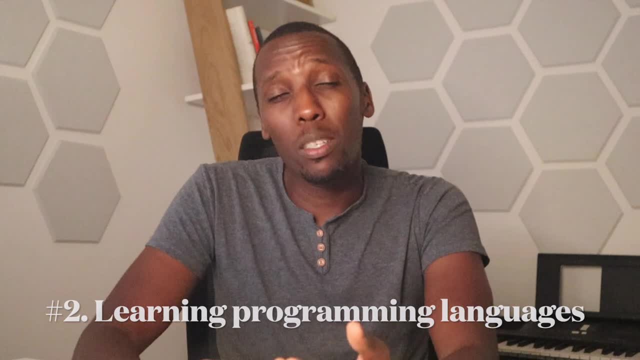 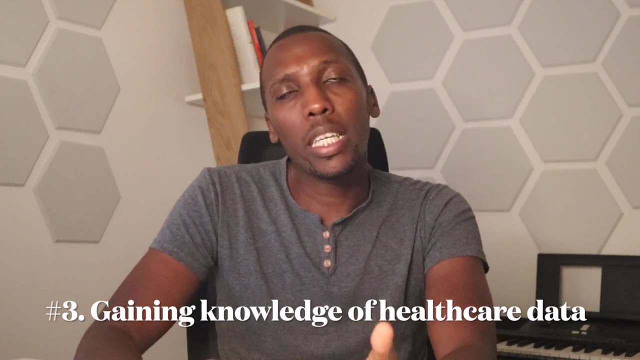 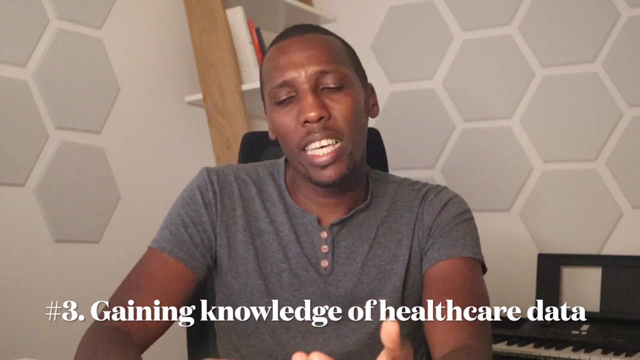 of becoming a health data analyst. with regards to learning, Gaining knowledge of healthcare data is also crucial for working as a health data analyst. So understanding the different types of data that are commonly used in healthcare, such as electronic health records, claims data and survey data, will help you to effectively analyze and 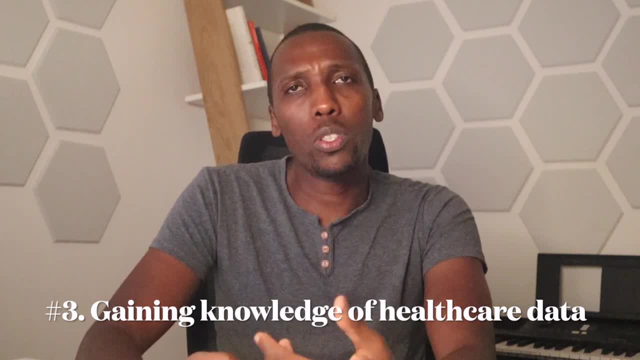 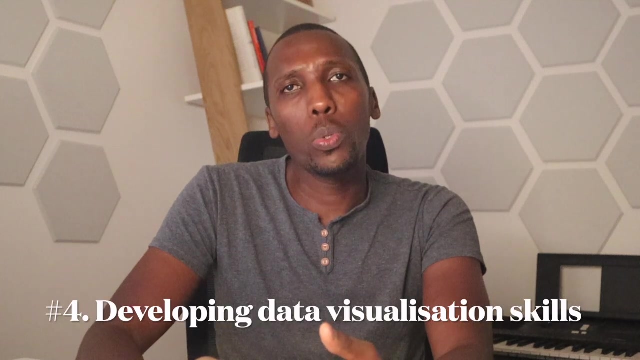 interpret data, And you can start by reading articles and books on healthcare data and its applications, So gaining knowledge of healthcare data is crucial for working as a health data analyst. The next thing that we are going to cover is developing data visualization skills. 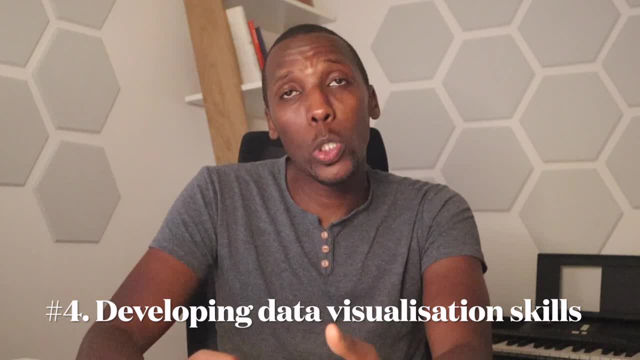 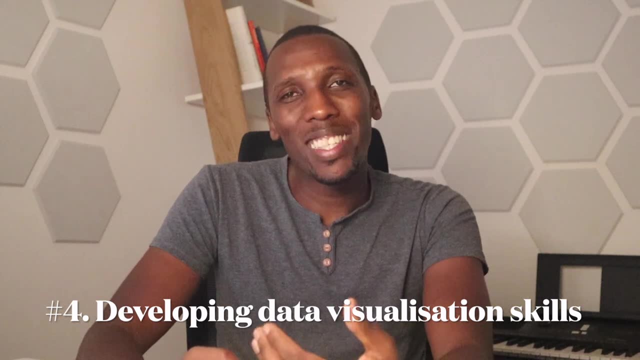 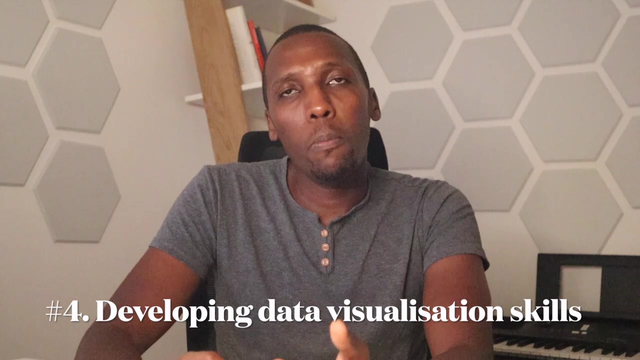 And it's important for health data analysts to be able to develop these skills, whether it's learning how to communicate through visualization tools such as Python or R, or even just using standalone visualization tools such as Power BI, So being able to communicate effectively your findings through those visualizations that you're. 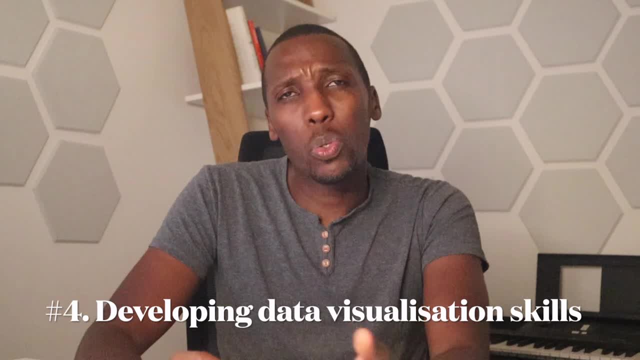 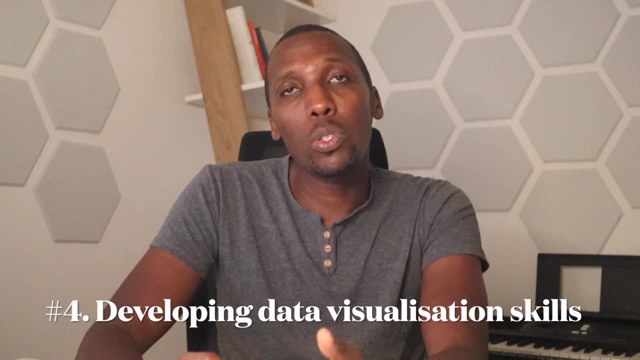 going to be creating, such as charts, graphs and maps, is crucial for presenting data in a clear and easy to understand manner. So you can start by learning those particular techniques that we've mentioned- the likes of charts and graphs and maps- and learning how you can be able to implement.